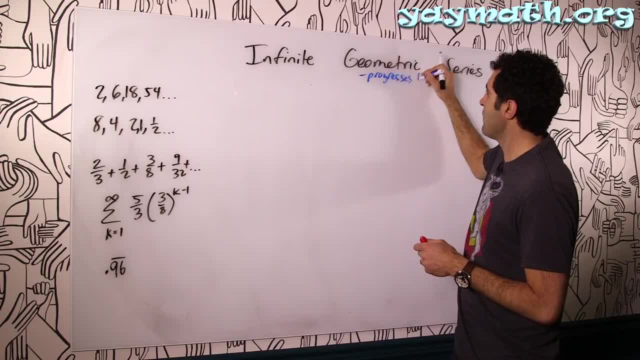 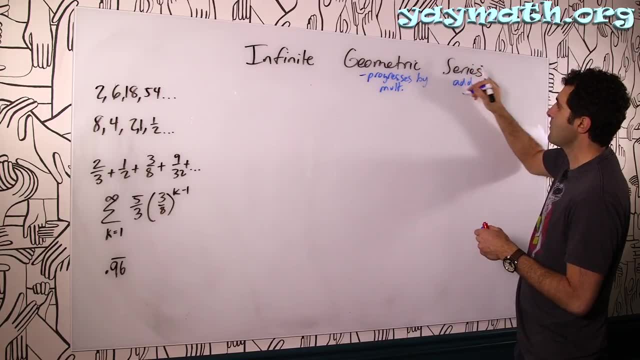 So this progresses by multiplication, And then we're going to add up the numbers, And then we're going to add up the numbers, And then we're going to add up the numbers And then we're going to add up all the terms. So that's the idea. So first let's understand. 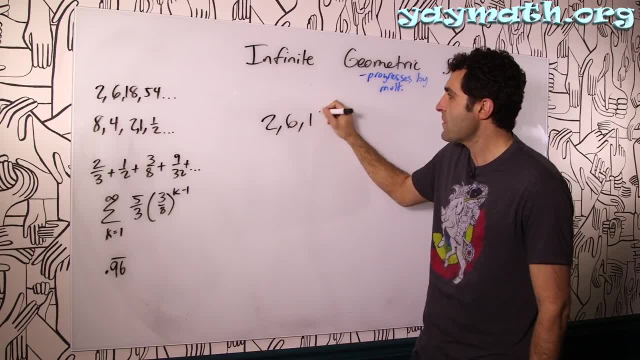 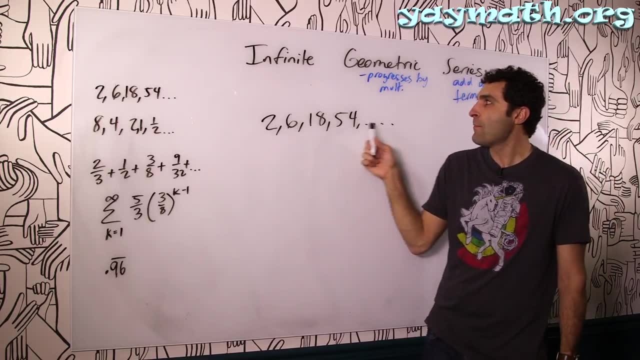 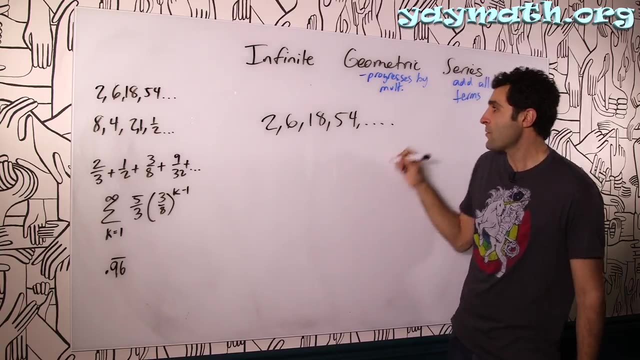 and get an example of a geometric sequence here. So we conclude: this is a geometric sequence because it does progress by multiplication: 2 times what is 6?, 6 times what is 18?, 18 times what is 54? It progresses by r equals 3, by a factor of 3.. The rate is 3.. 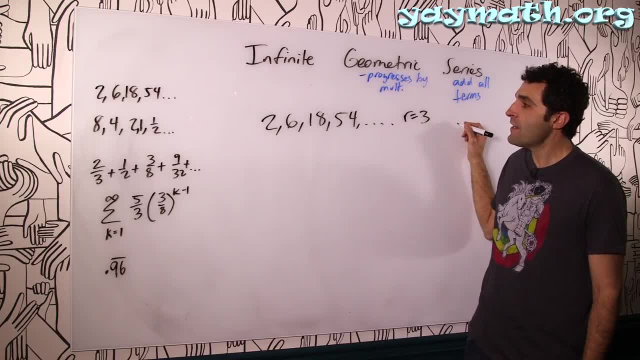 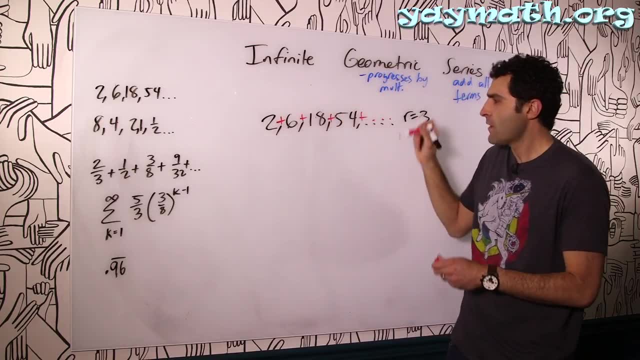 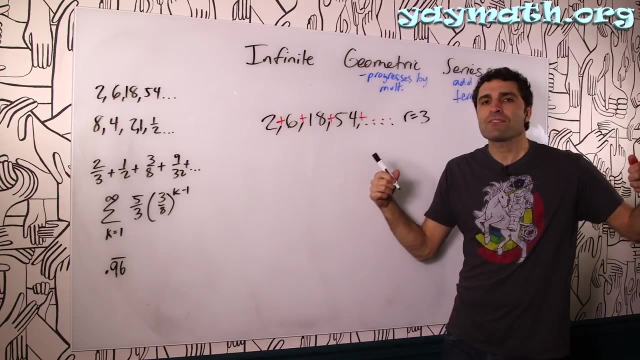 The question is, if I continued on to infinity and I added all these up all the way up to infinity, would that even be possible, is the question, And the answer is no, because I would never be able to get a fix on what that total sum was if it kept going on and 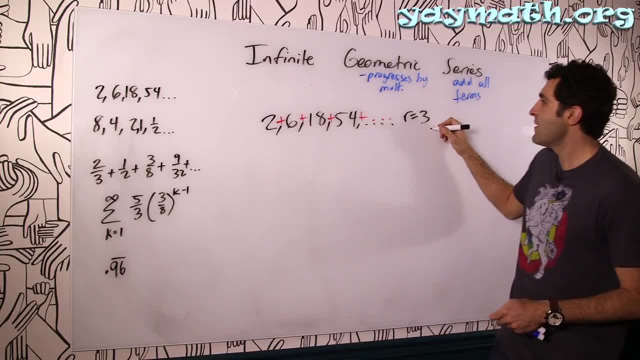 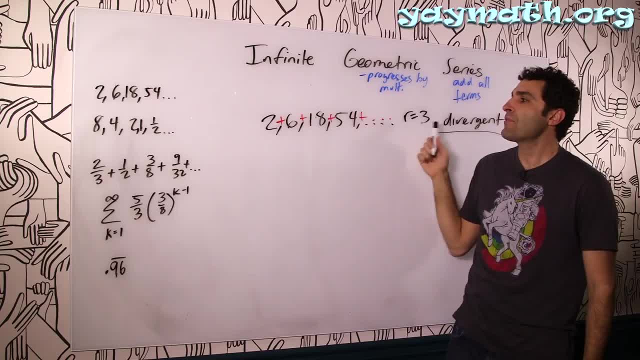 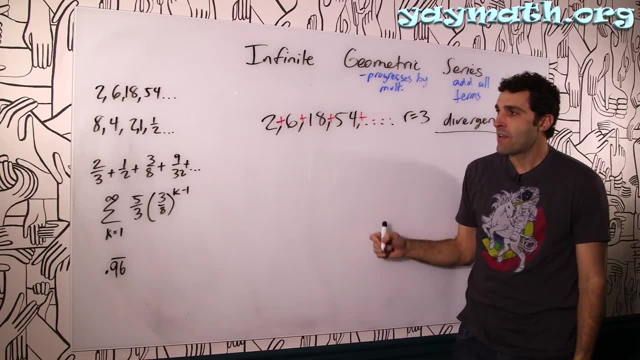 So it's like it just goes and goes and gets away from us. We can't really add up this particular sequence because it just gets bigger and bigger and bigger and we'll never know what it is. But what if the sequence was like this: 8,, looking at it, 4,, 2, 1,. 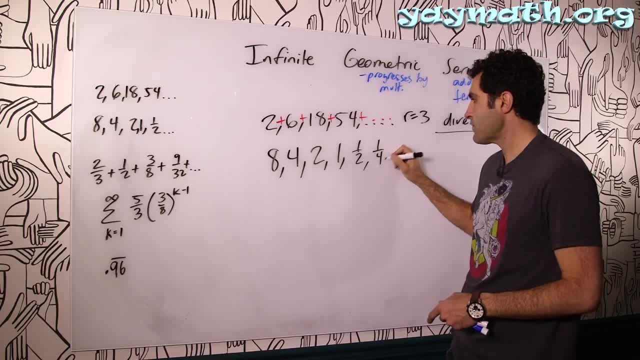 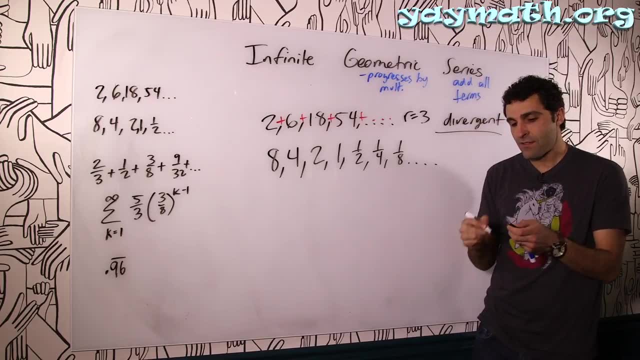 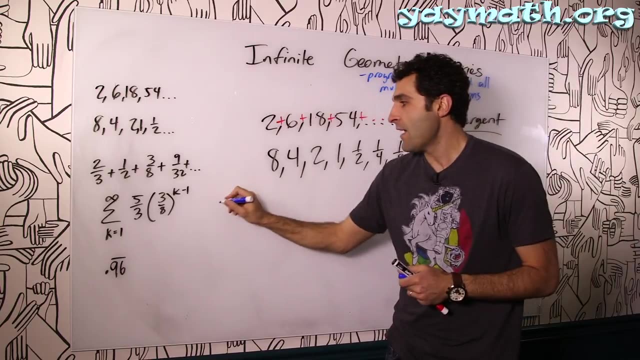 1 half. Yeah, let's go further: 1 fourth, 1 eighth and so on. Now, if you look closely, this is also a geometric sequence. It does progress by multiplication. In this case, we're multiplying by 1 half. We could even see that 4 over 8 is the same as 2 over 4 is. 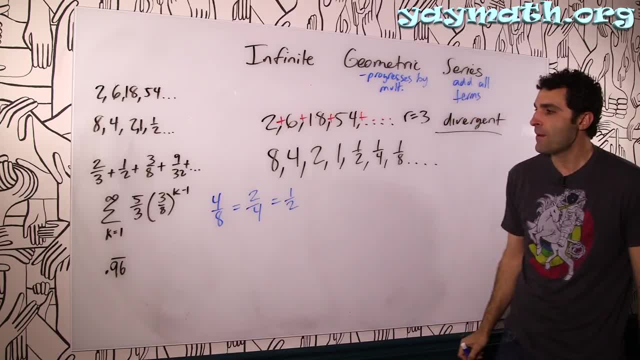 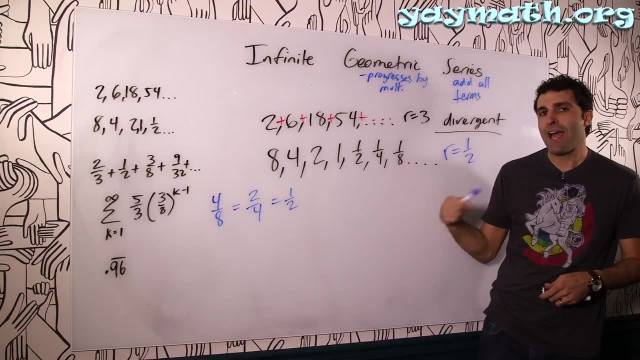 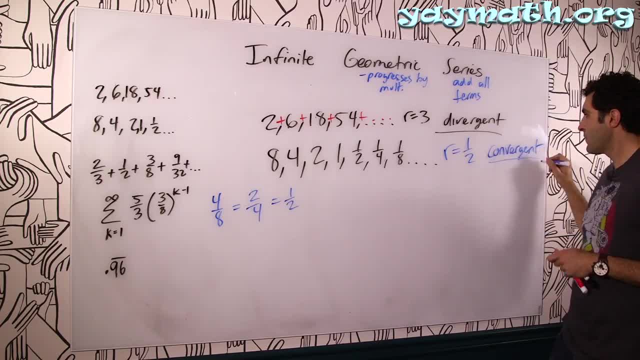 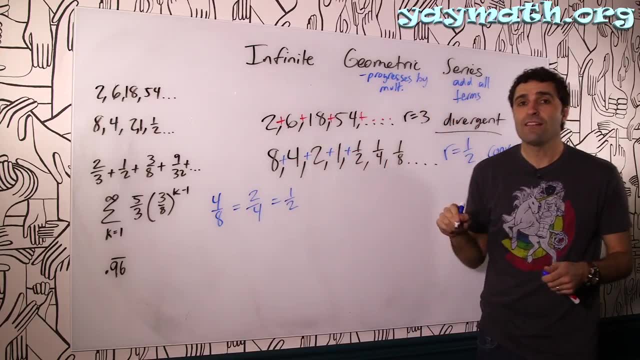 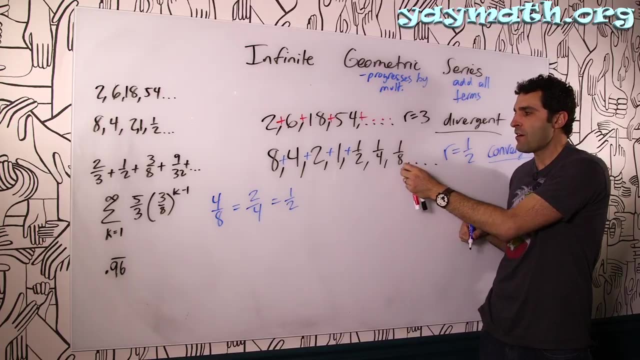 on some value, So what converges to some value. And if you were to add all these up, you would actually get a number. It would actually sort of peter out and fizzle out and go away. It basically goes closer and closer to 0.. So if you keep multiplying this by a half and a half and 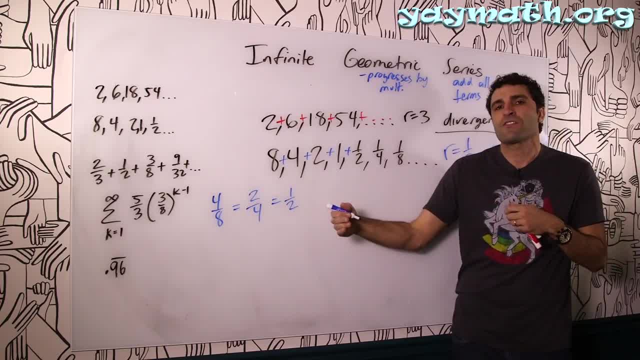 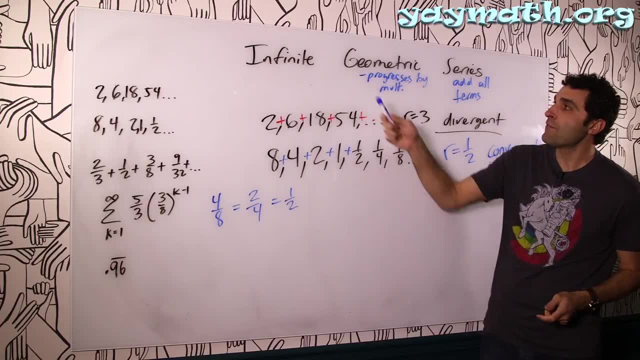 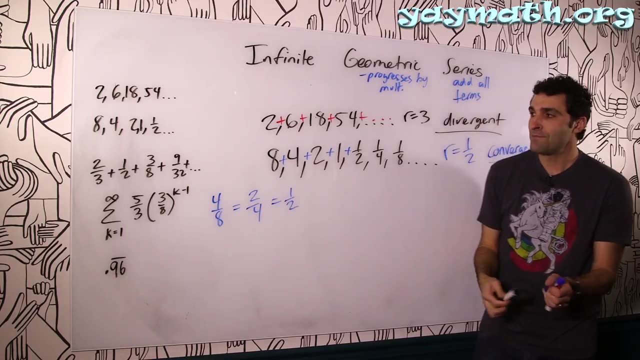 a half, it would just get smaller and smaller and smaller and then eventually it sort of just stops essentially, and you could add them up and actually get a value. okay, So that is what an infinite geometric series is, Remember. in this sequence it goes on to infinity and we add them all up. Let's give 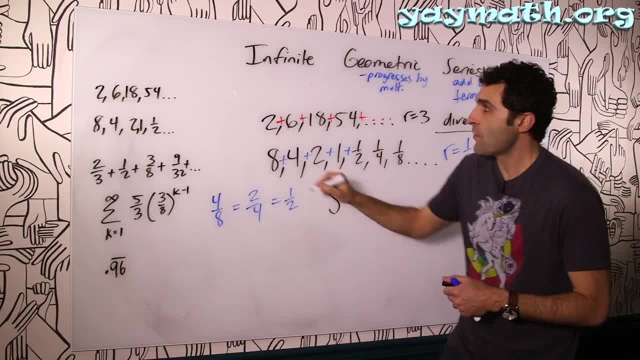 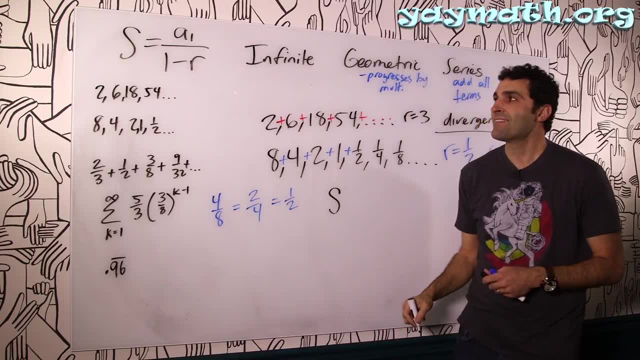 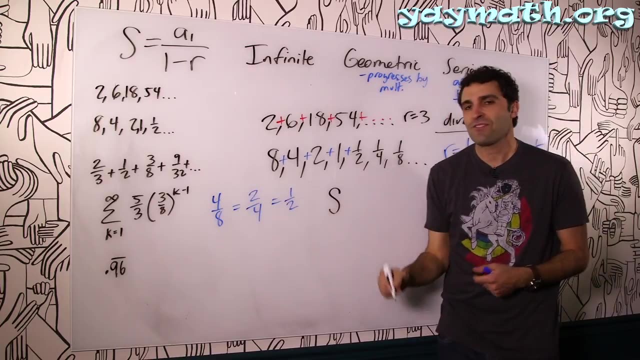 you that formula, The sum. let's put it over here as well: the sum equals first term over 1 minus r. That's it. It's kind of amazing: First term over 1 minus r is the sum of all these terms added up to infinity. It's just crazy to me how simple it is. All right, let's. 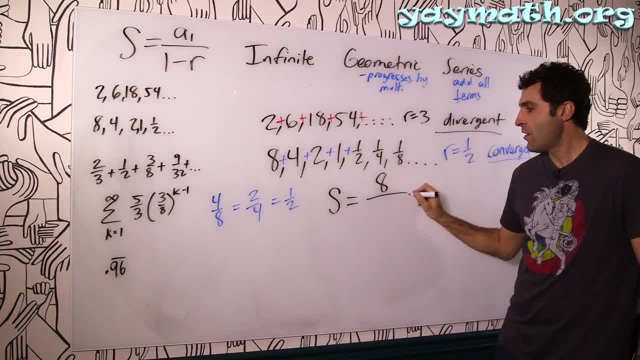 prove it: First term: 8 over 1 minus r. First term: 8 over 1 minus r. First term: 8 over 1 minus r. Mr 1 minus r in this case is 1 half, So this becomes: 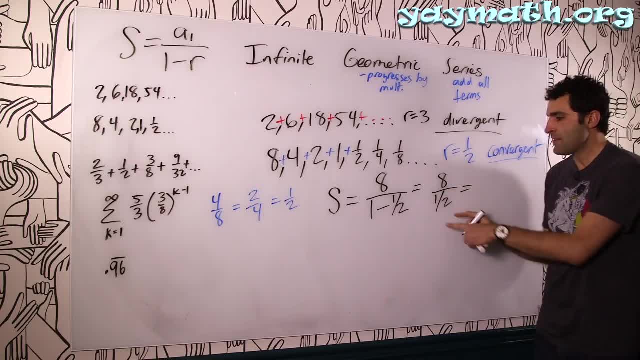 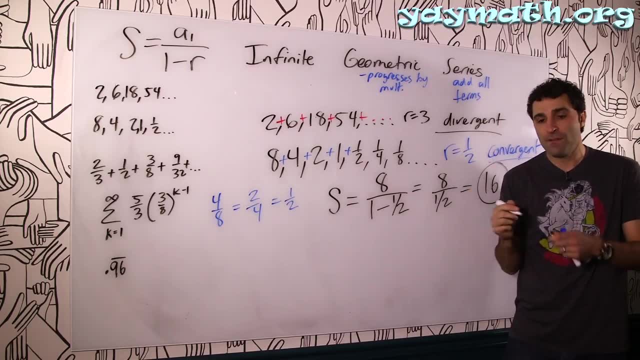 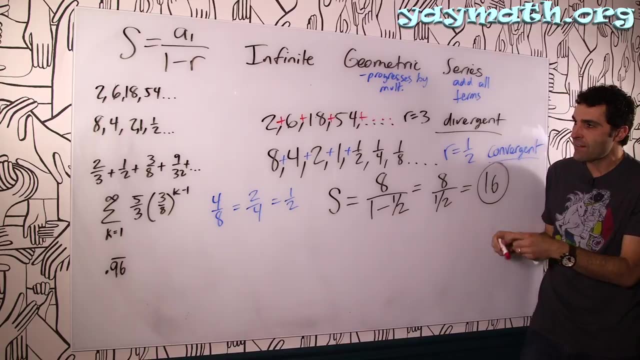 8 over 1 half. How many times does 1 half go into 8? 16.. There it is. That's the sum of this infinite geometric series. and you know what's even more fun? I noticed that you could find the 16 hiding inside here. Check it out. 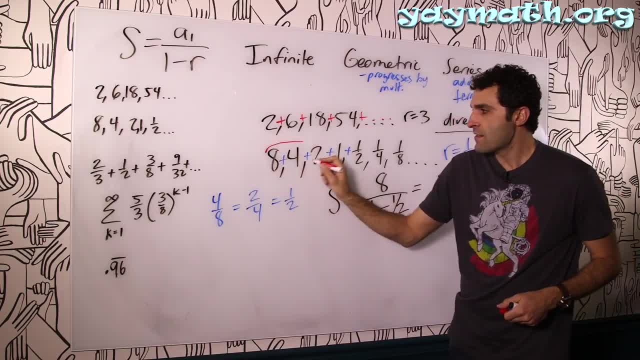 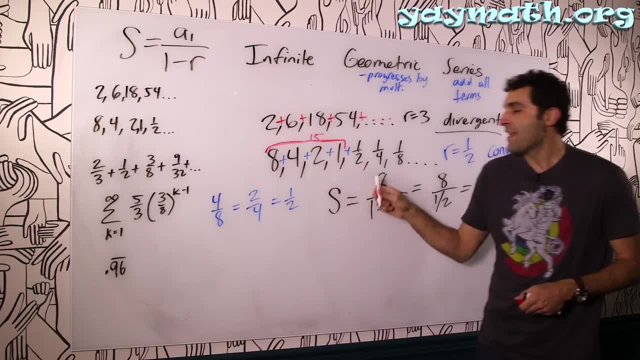 8 plus 4, that's 12.. This is 14 plus 1. So this is like 15 right here. And then you have all the chunks, all the fractions: One half plus a fourth plus an eighth. keep adding, adding, adding. 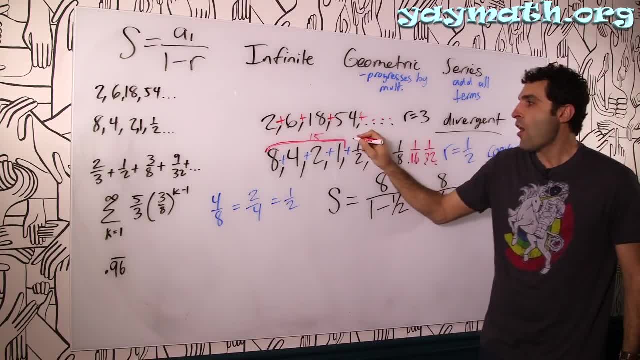 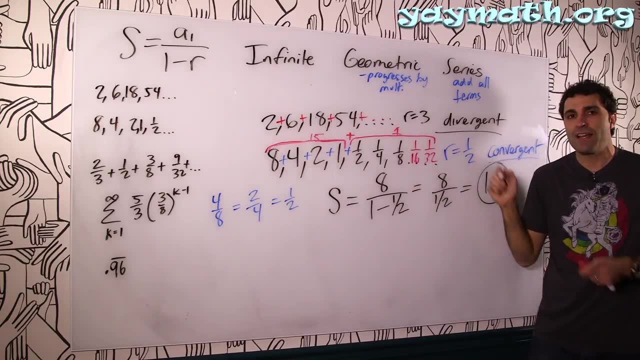 One over 16,, one over 32, keep adding them up. All that stuff would basically add to one over time. And there's your 16 right there hiding inside. All these numbers add up to 16, that's all it is. 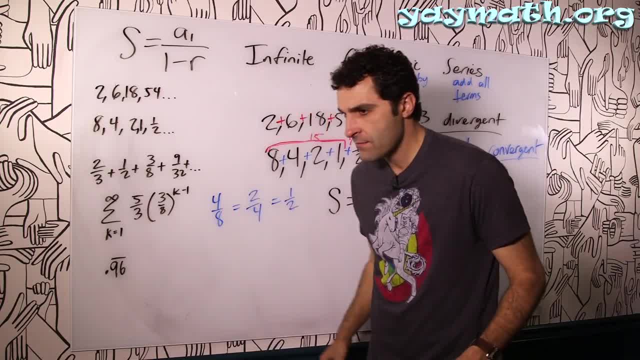 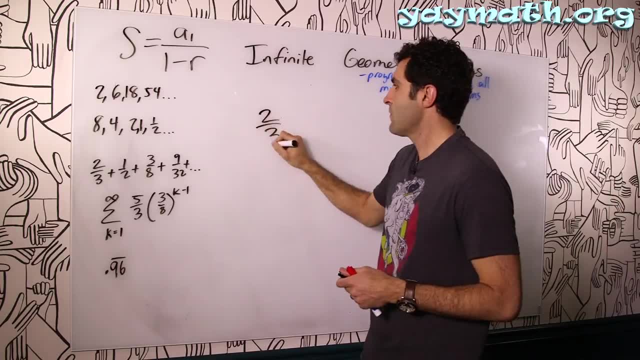 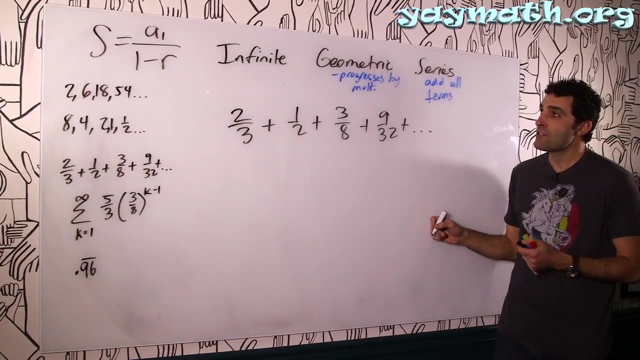 I'm gonna erase it and add it. oh, there it is. Let me get this bag out of the way. Okay, So this one looks a little intimidating at first, but we have to first see whether it's geometric, So let's do the test. 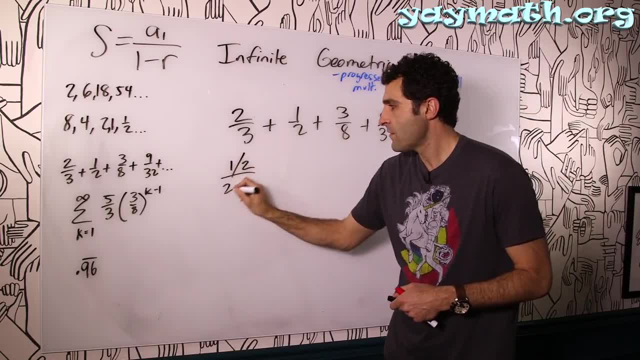 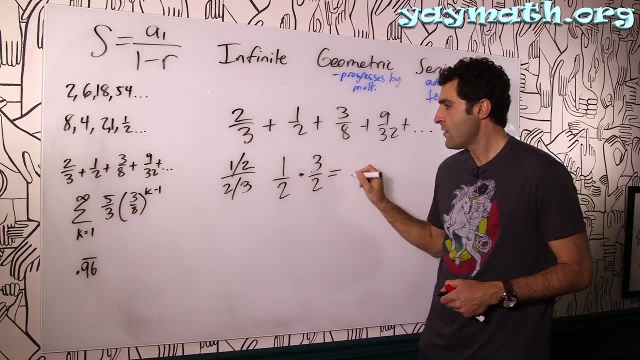 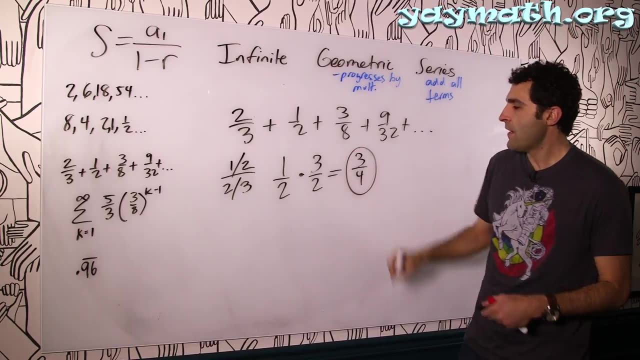 We divide the second term by the first and see what that is. That's the same as one over two times three over two. That works, which is three over four. So if this is geometric, we should get the same rate for dividing the third term into the second here. 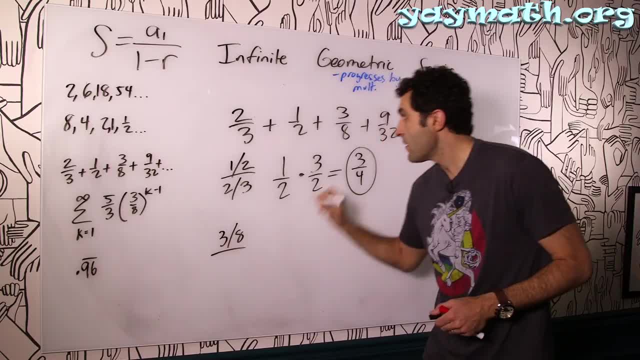 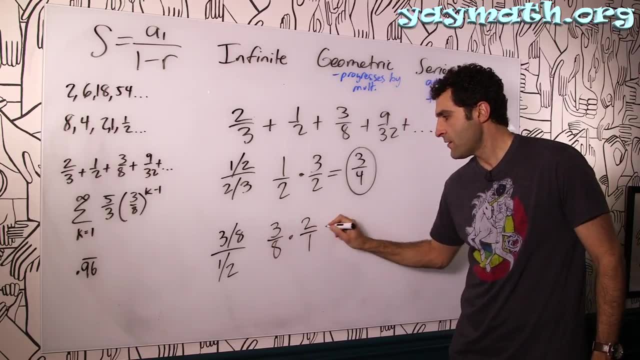 or over the second. So that would be three over eight divided by one half. We're just trying to get the rate here which is the same as three over eight times two over one, which indeed goes: this is four. this is great. 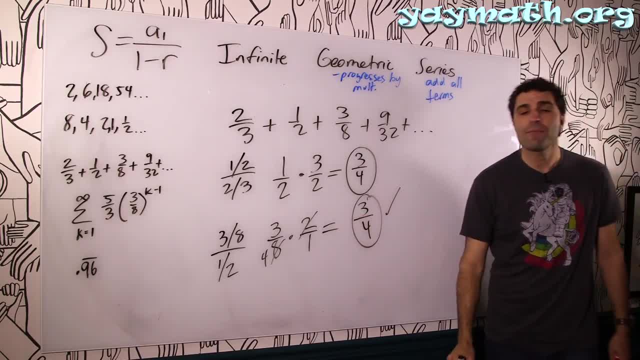 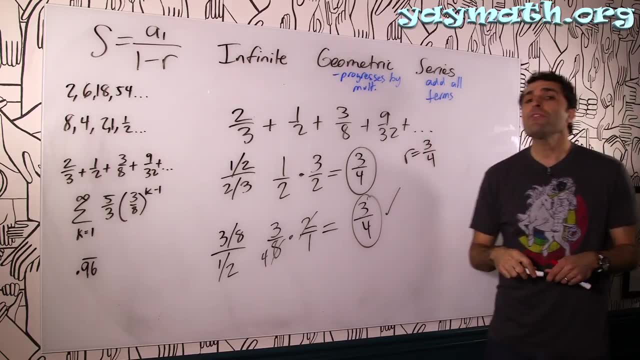 three over four. yes, so we're confirming- Okay, We're confirming- that this is a geometric sequence in which the rate of growth is three over four. Now here's the giveaway: How do you know if a series will be convergent or divergent? 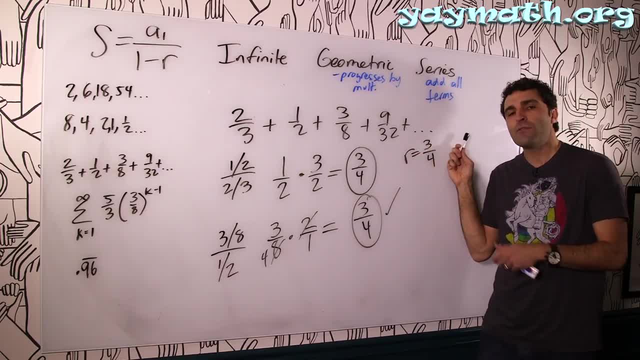 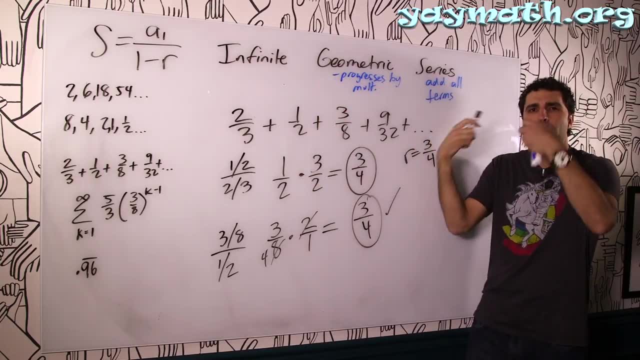 How do you know if this will fizzle out eventually and go closer and closer to zero, such that you can add it up, Or if it won't fizzle out and it will just become bigger and bigger and bigger, and then we will not be able to get the infinite sum. 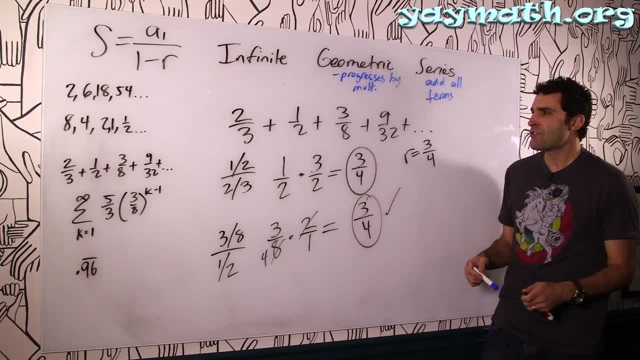 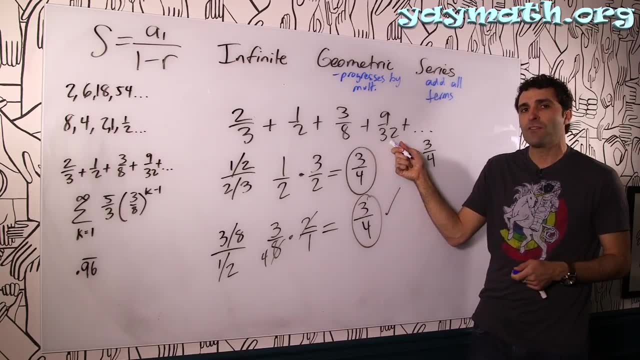 How do you know right? The answer is pretty logical once you wrap your head around it. Would it make sense that if this number continues to get smaller and smaller and smaller, eventually it'll be convergent, it'll close in on a specific value? 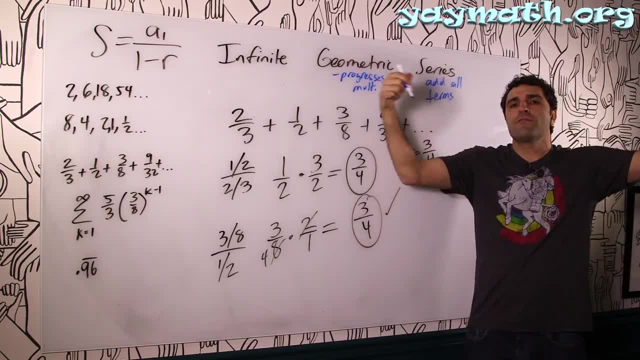 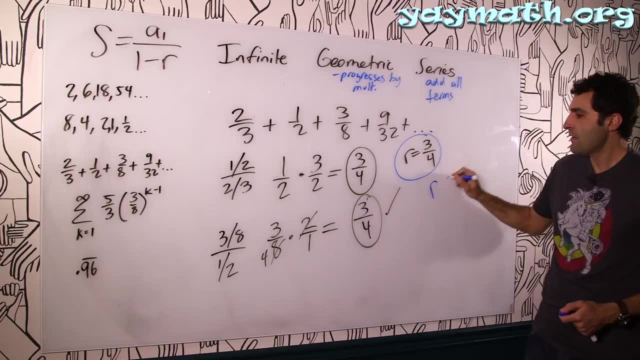 Versus. if this number gets bigger and bigger and bigger, it'll just go to infinity and explode and we would never be able to get a grip on it. So this value here needs to basically be less than one. If you multiply by something less than one, then this value 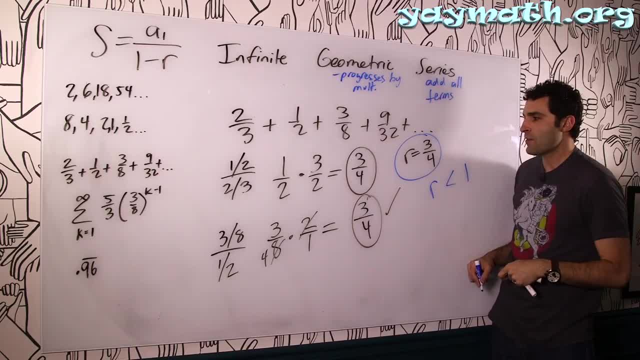 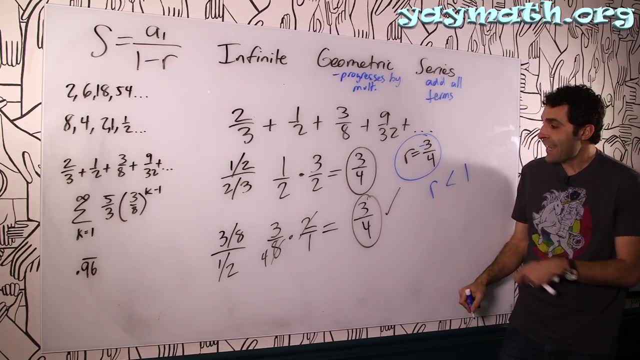 the sequence will continue to get smaller and smaller. Not only that, it would be okay if r was actually negative in that case. So it's okay to multiply by a number that's negative. but basically you wanna say it like that. 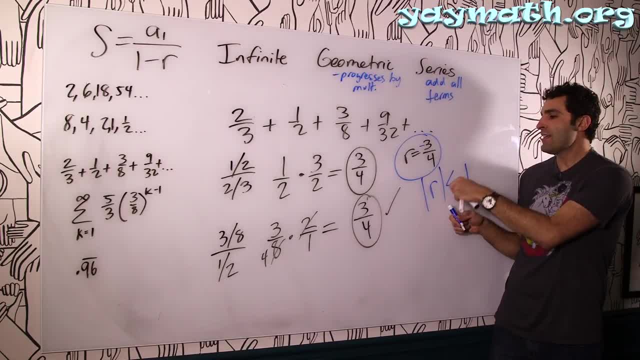 So the absolute value of r, whatever that r is- needs to be less than one, because that will make these guys get smaller and smaller and smaller. eventually they'll fizzle out and go to zero, and then you could add up those terms on the line. 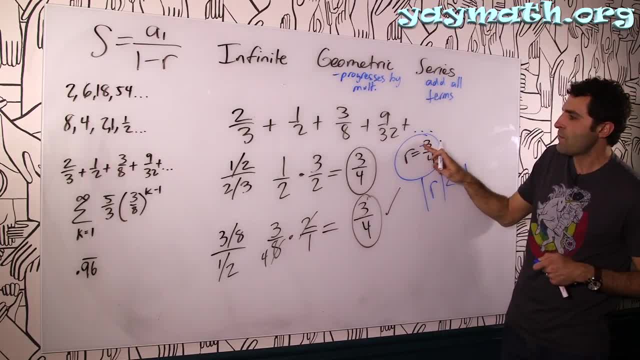 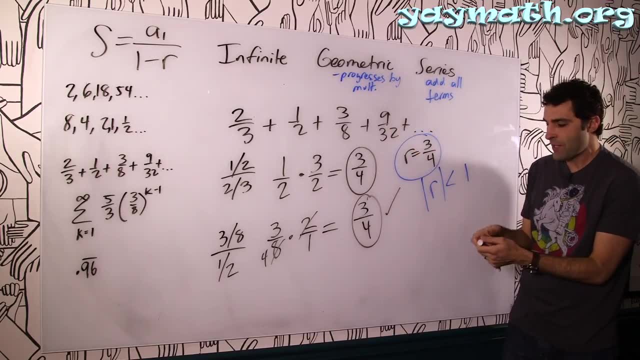 I hope that makes sense. So as long as your r value, your rate, is less than one, you're in good shape, And we are. Let's find out what this infinite geometric series would be, what it would add up to. 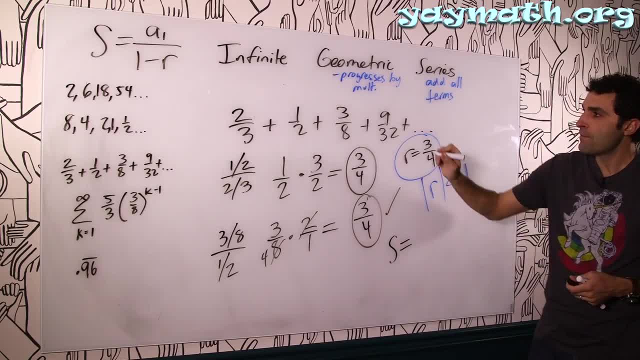 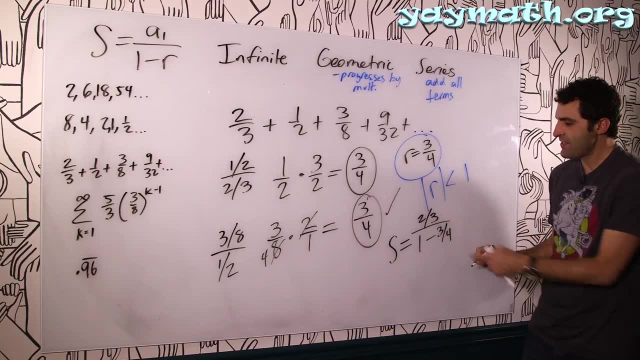 Formula S equals, first term, two over three over one. minus the rate is three over four. This is it. this is the sum of infinite terms. It's crazy to me. Let's find out what it is. This is two over three. 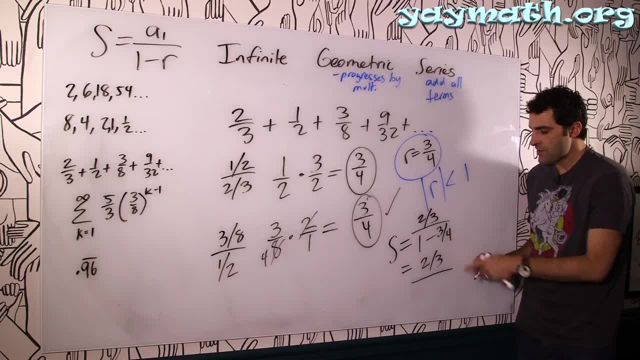 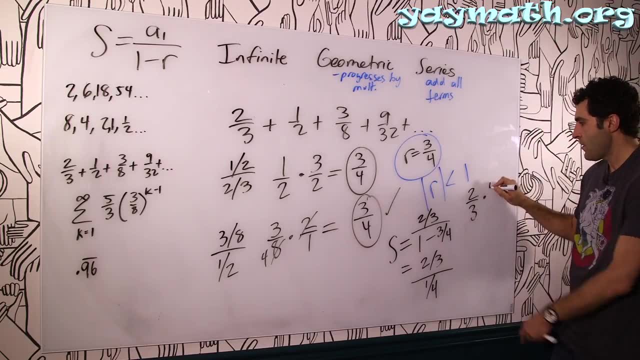 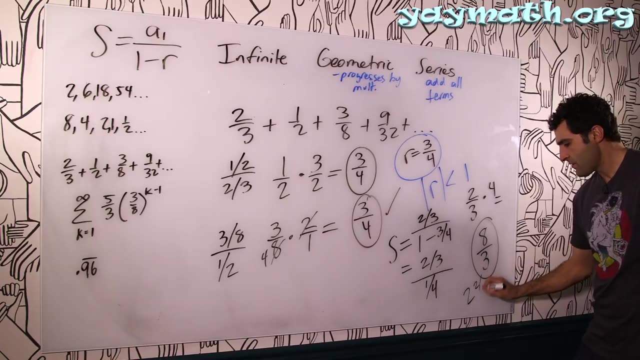 Over. this is four. fourths minus three fourths is one fourth, All right. Which is the same as two over three times four, which is eight over three. Wow, Eight thirds. Two and two thirds, All these numbers added up to infinity. 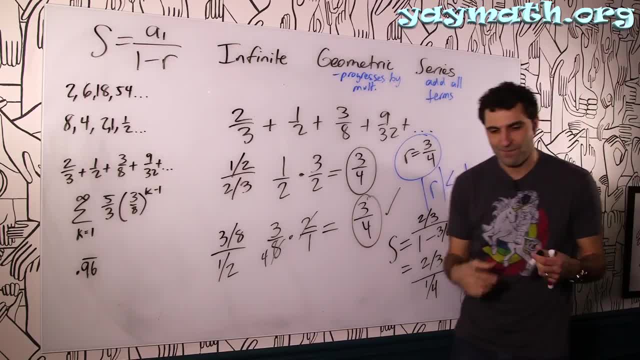 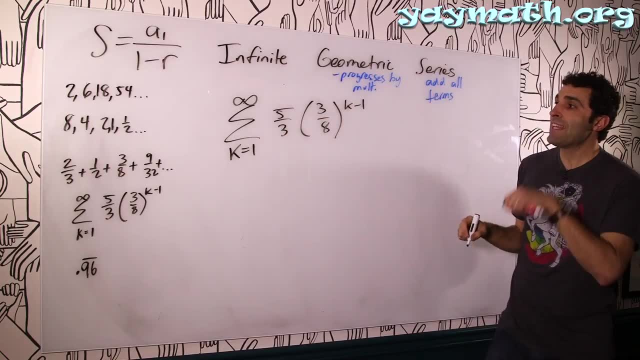 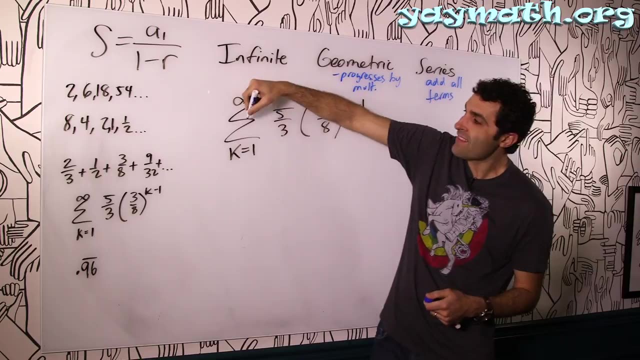 is nothing more than two and two thirds. How about that? It's amazing, Okay, Mm. So here we have an infinite geometric sum as well. You'll see, this is the symbol sigma Symbol, the Greek symbol for sigma stands for sum. 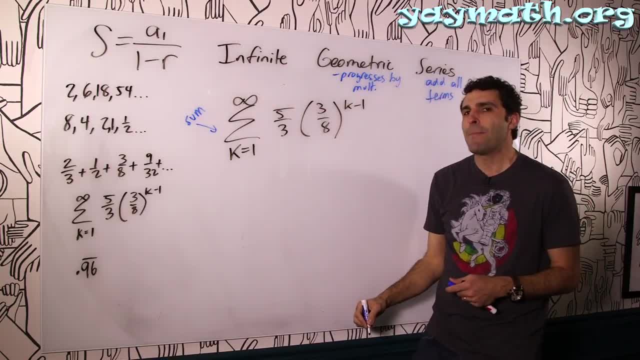 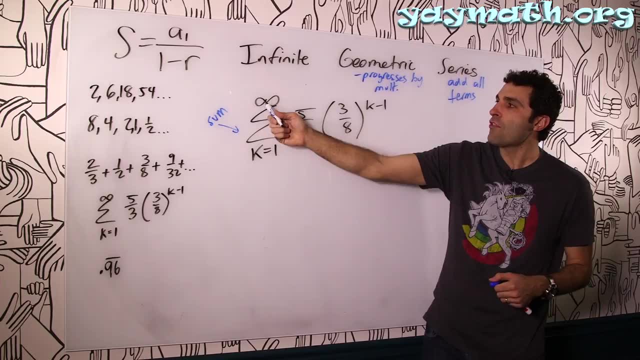 That's a lot of S's. The Greek symbol for sigma stands for sum. That's a lot. So you'll notice that the sum ranges from when k is one all the way to when k is infinity. okay, So that's the giveaway, that it's infinite. 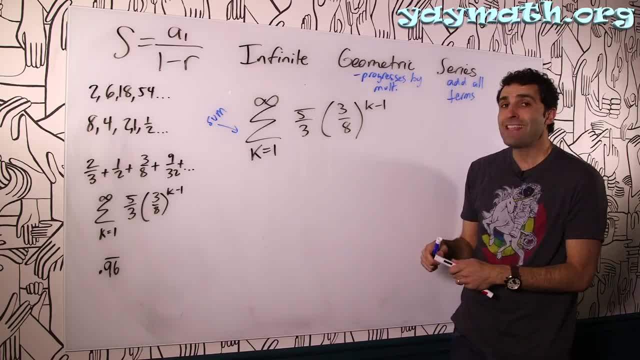 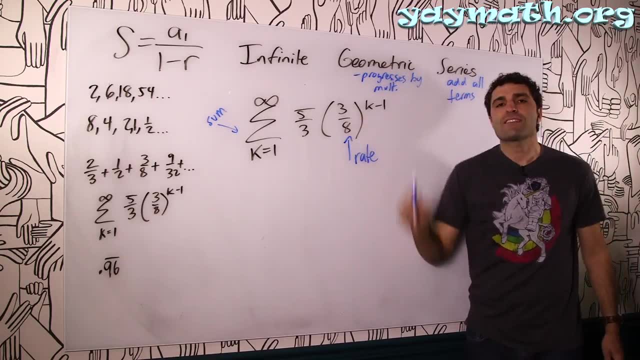 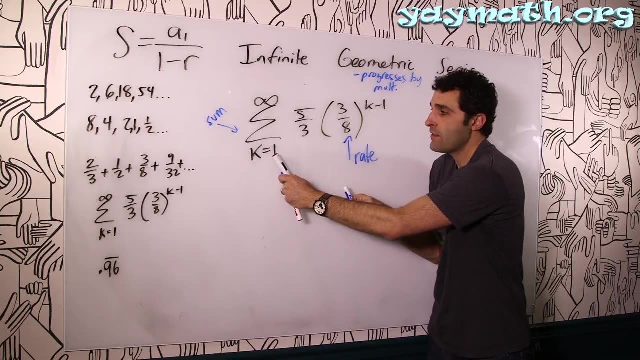 We ask ourselves: can this be done? And the answer is yes, For the simple fact that our rate of growth right here is a fraction, that's less than one. That's good news, And we also can get our first term. The first term is when k is one. 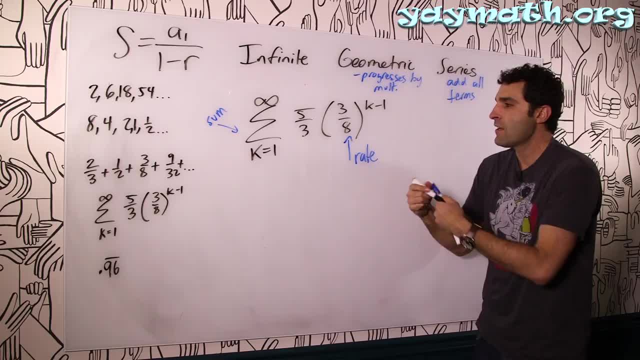 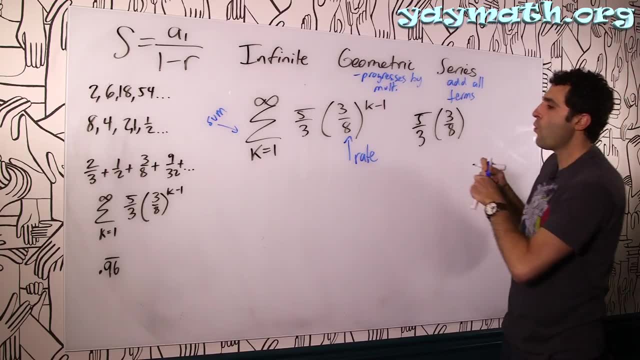 And when k is one, we throw in one over here. Let's see what would happen When k is one. we would get five thirds times three over eight to the one Mm Minus one. Again, the first term is when k is one. 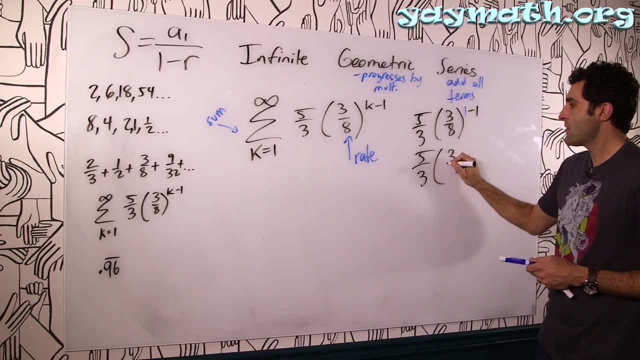 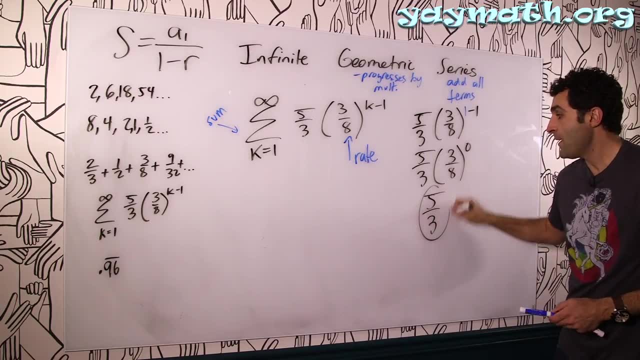 One minus one is zero. That's five over three times three over eight. to the zero. This is the number one, So that becomes five over three. A big giveaway for anything in sigma notation like this When you see geometric sequences as such. 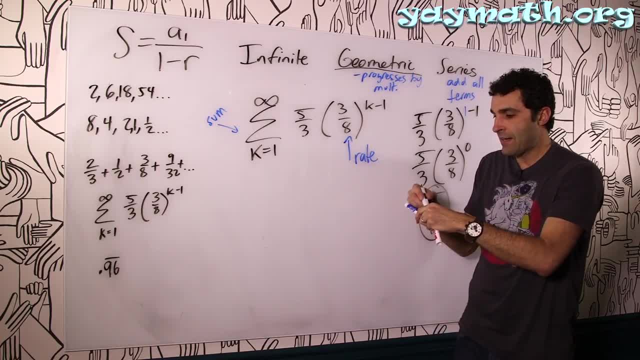 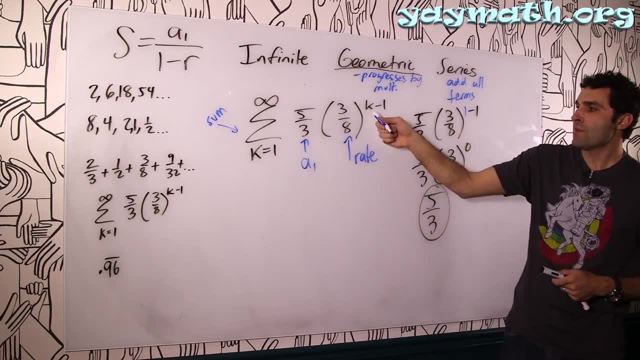 that the rate is hiding inside here. That's raised to the power And inevitably this becomes the first term. It's kind of amazing. You could sort of decode it right in there, Because when k is one, this thing goes away. 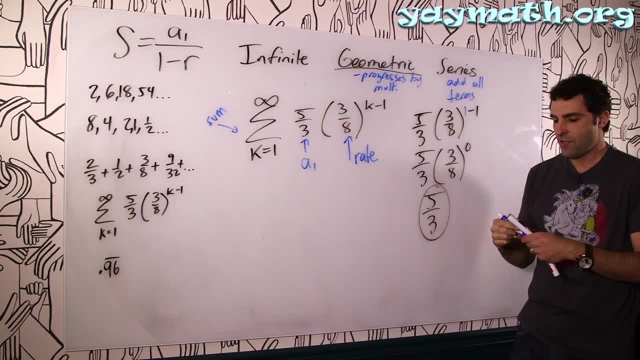 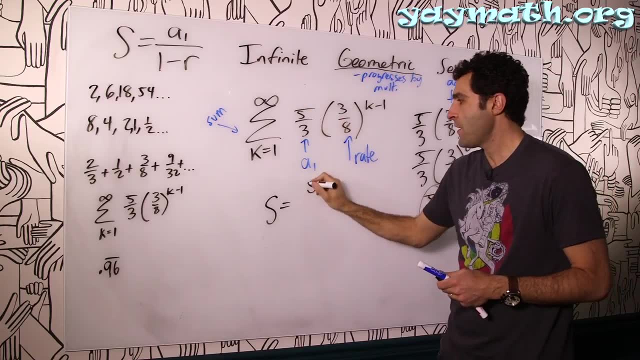 That becomes the number one times five thirds. There it is, That's the first term. Let's go ahead and get this infinite sum. Sum equals the first term: Five over three, One minus the rate. What's the rate? None other than three over eight. 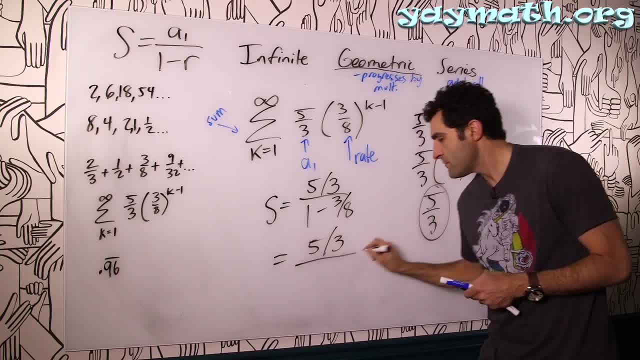 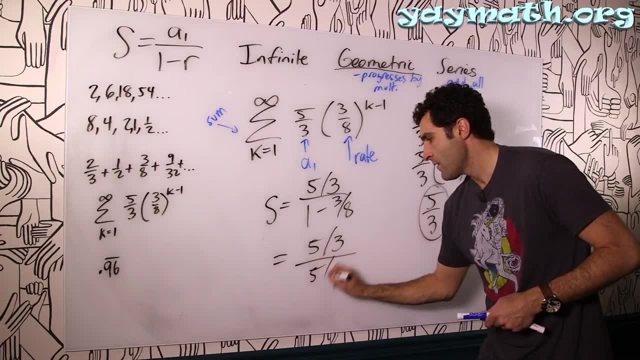 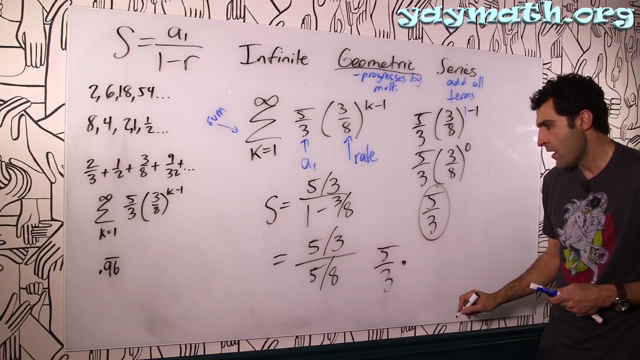 Doing it and doing it, and doing it. well, Uh, eight over eight Minus three over eight is five over eight. Ooh, this is nice. So we're going to get five over three times eight over five Knees go. 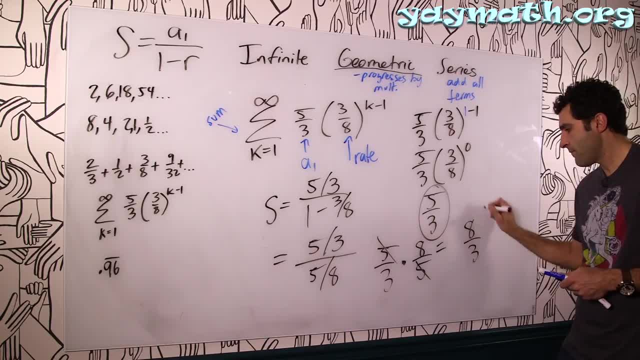 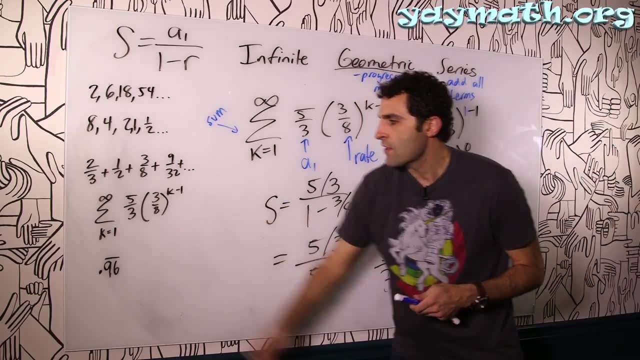 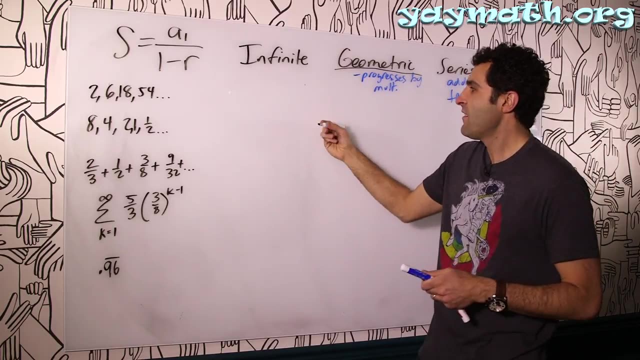 Boom, boom And we get eight over three again. All right, that's for this particular one. All right, that's a coincidence from the last problem. Right, because you see different starting terms. Okay, one more Now. admittedly, when I was prepping, 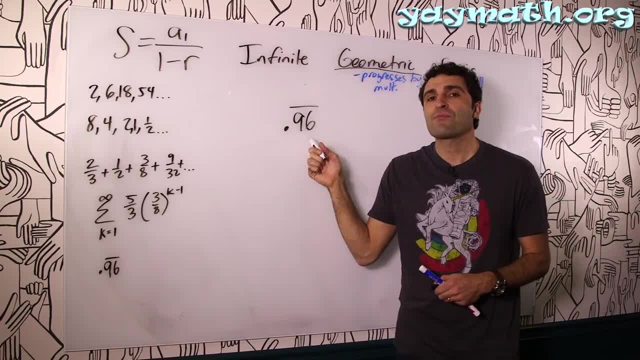 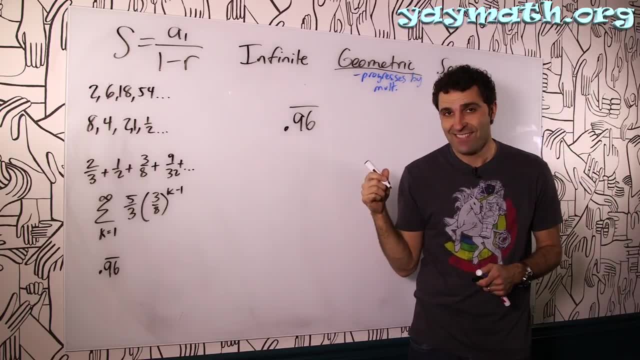 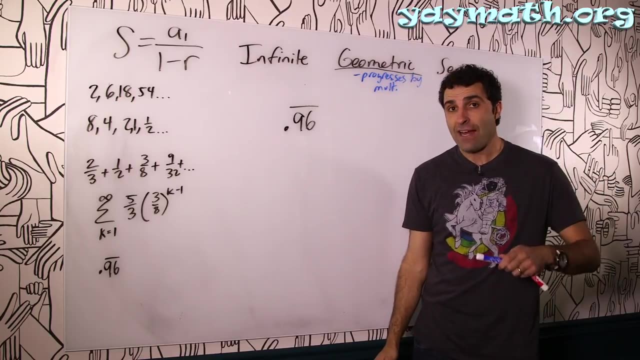 for this particular lesson, I learned that you can express this as a fraction using infinite geometric series. I learned this last night. okay, I literally learned this last night. There are ways to express .96, repeating as a fraction using other algebraic terms or other algebraic methods. 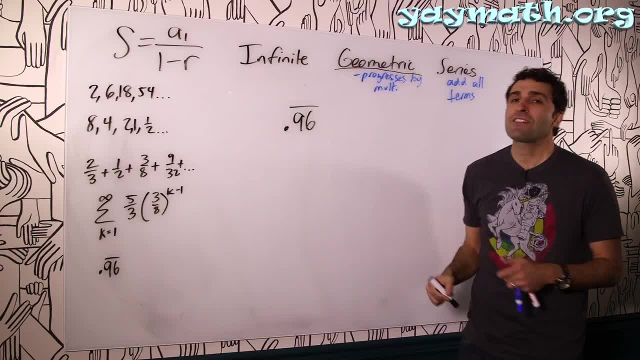 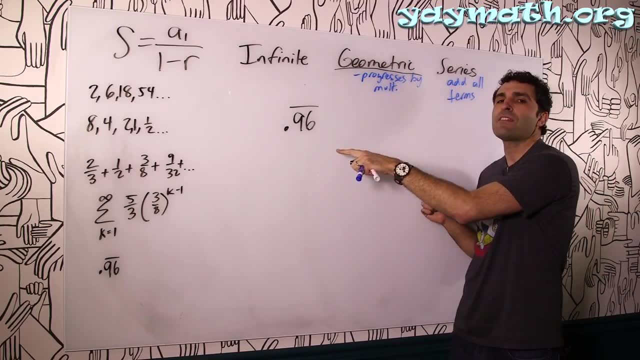 But there is one way to do it. But there is a way to do it with infinite geometric series and we're going to do that now. It's kind of pretty amazing the way it works. Okay, so this is an infinite geometric series. 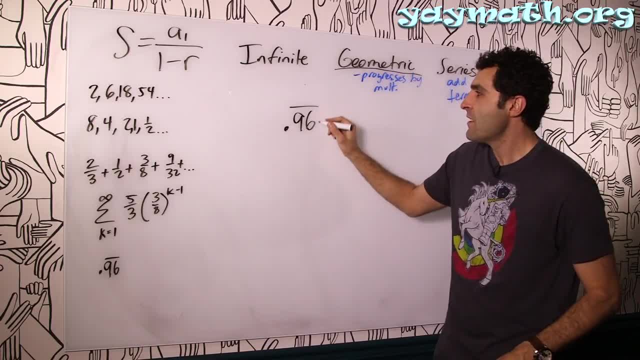 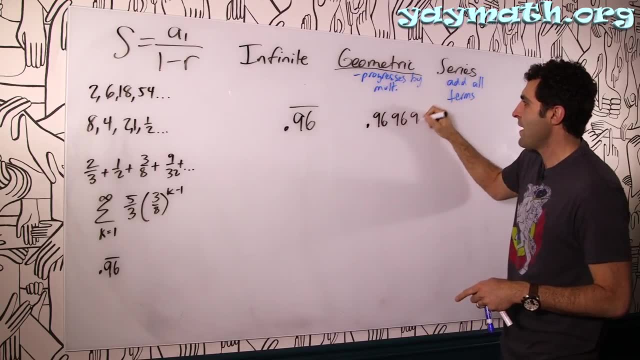 and I'll prove it to you, Because this can be expressed as: again, this is .96, repeating That's what this bar means. So it's like this: .96969696, on, and on, and on, and on. All right. 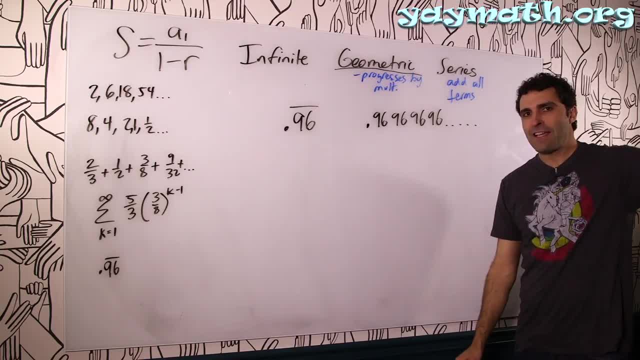 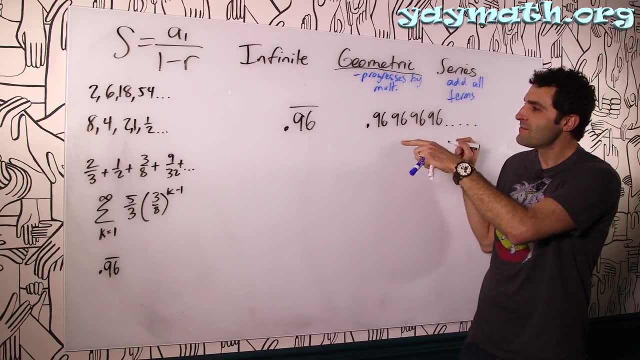 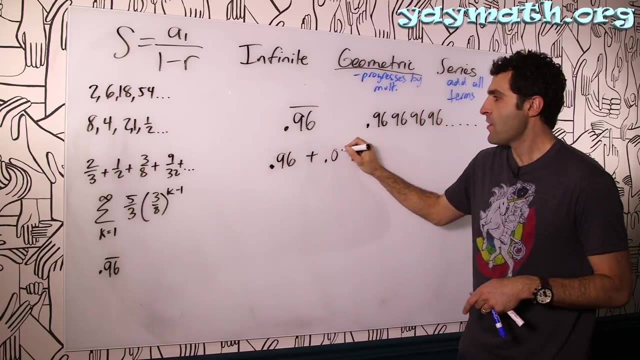 So class of 96, Wildcats. Oh my God, I can't do shout-outs for myself anymore. I'm dating myself hardcore. So this is the infinite geometric series. I'll show it to you. That means it's .96 plus .0096, you see it. 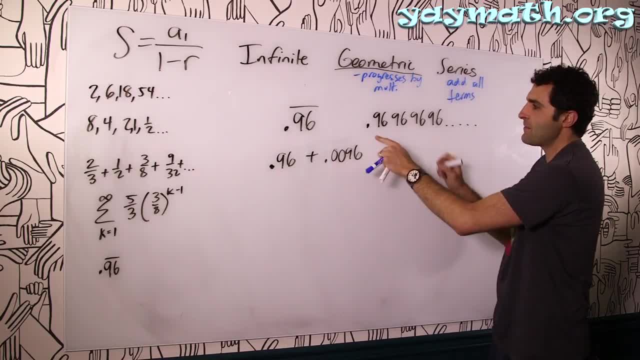 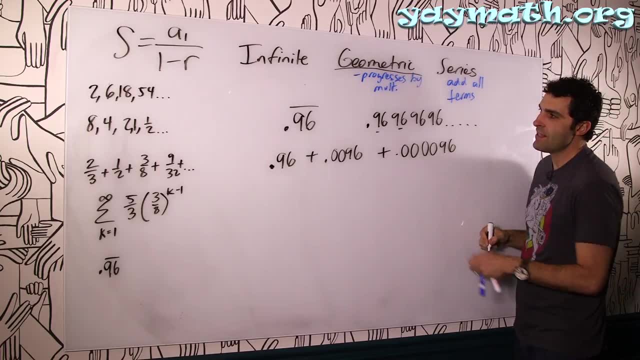 That's where this 96 was. Now I have four decimal places taken into account plus .000096,. see that. So I have 96 here, Then I have 0096 here, Then I have four decimal places And then another 96 here. 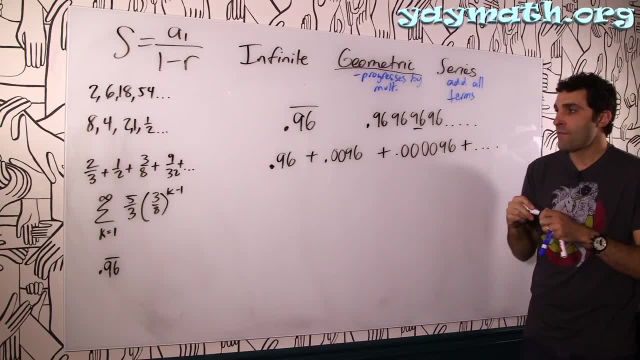 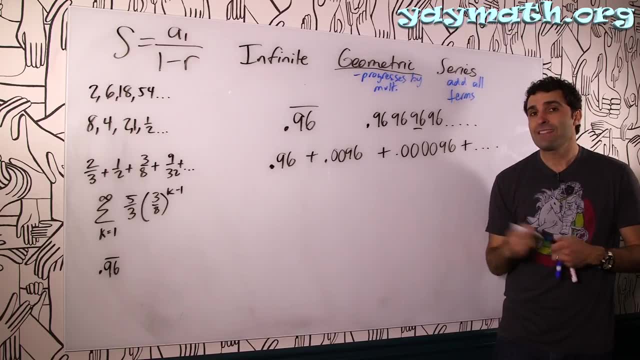 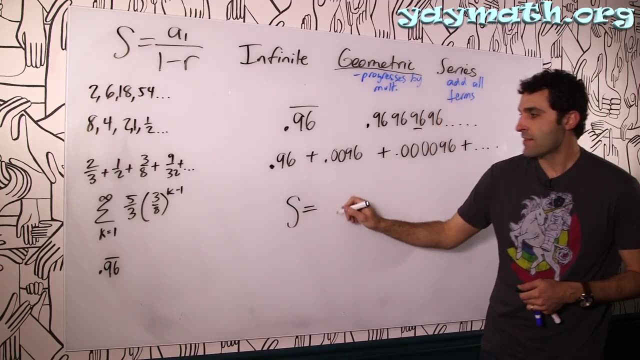 And I just keep adding to infinity, don't I Right? So if that's the case, you can represent this using infinite geometric sequences. Let's see if we can get the formula. The sum equals the first term, .96.. One minus the rate. 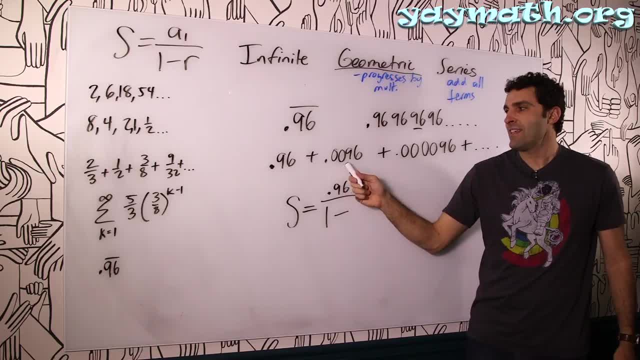 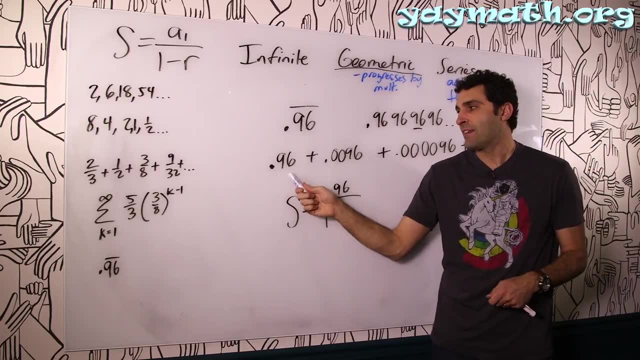 Now, what's the rate? How do you go from here to here? How do you go from here to here? What do you multiply by? What do you multiply .96 by to get .0096?? You see it, You see how the decimal place moved over twice. 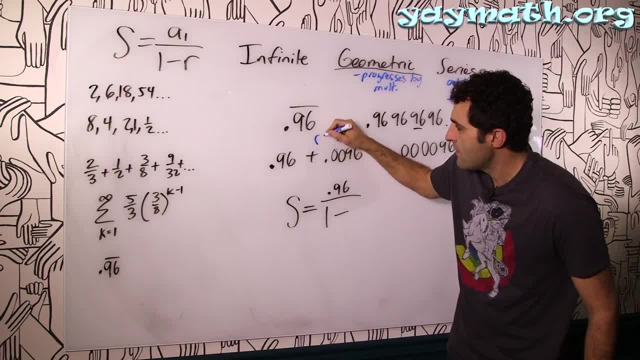 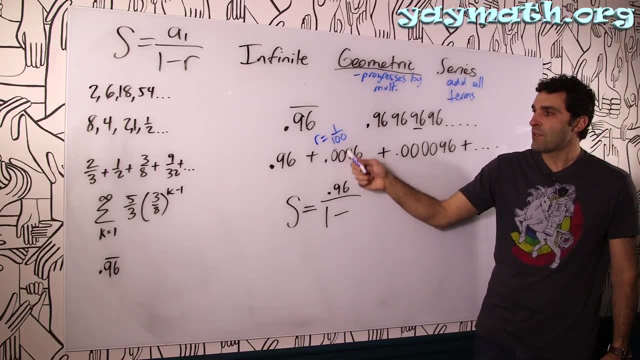 One, two. That means you multiplied by one over 100.. Right, You multiply by one over 100. In other words, if you multiply by one over 100, or you, it's sort of like a a percent thing. 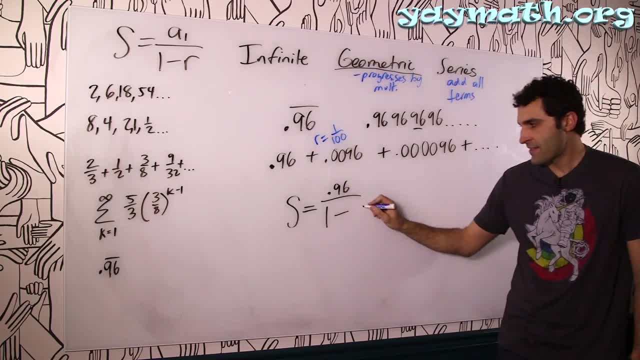 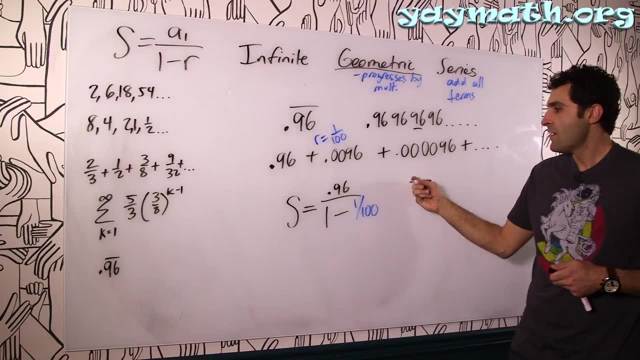 you move the decimal over twice for these two zeros. So that's the rate: one over one over 100.. All right, So now we can simplify this, and we're done. So for funsies, I want to turn this all into fraction land. 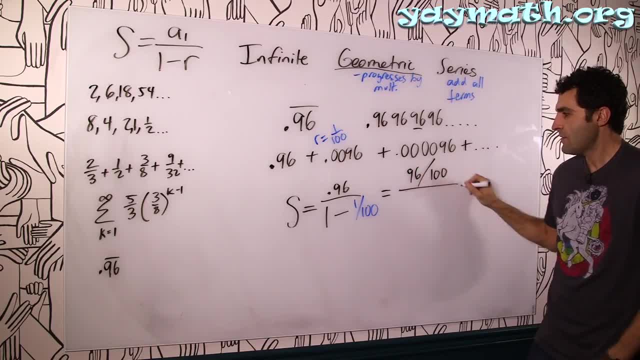 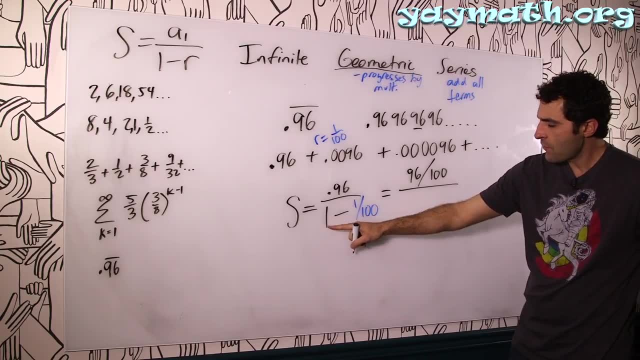 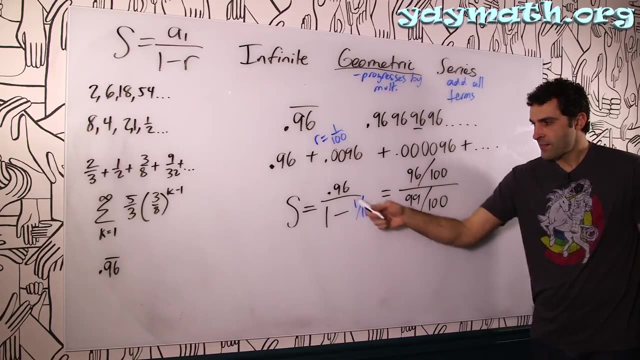 So this would be 96 over 100.. That's what .96 is. This would be 100 over 100, minus one over 100. That's 99 over 100.. Okay, that's what that is. That's one minus a hundredth would be 99 hundredths left. 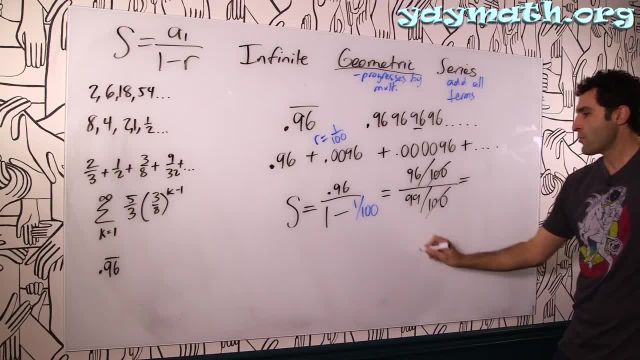 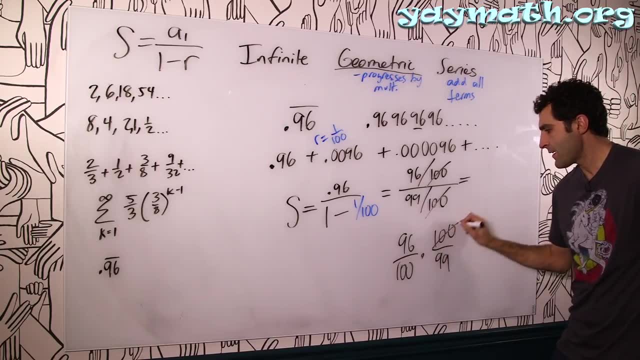 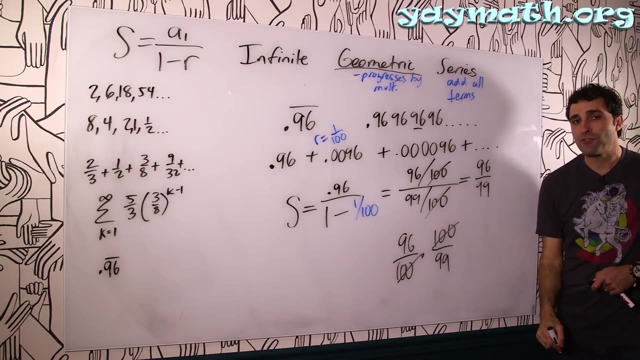 So if you look closely, you know that you could do this. I'll prove it to you: 96 over 100 times 100 over 99, gaon, gaon And you're left with 96 over 99.. This simplifies by a factor of three.